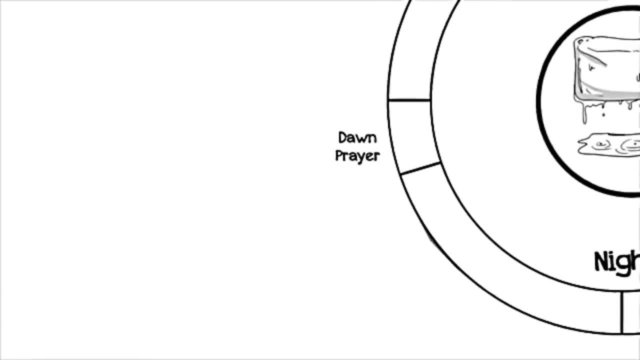 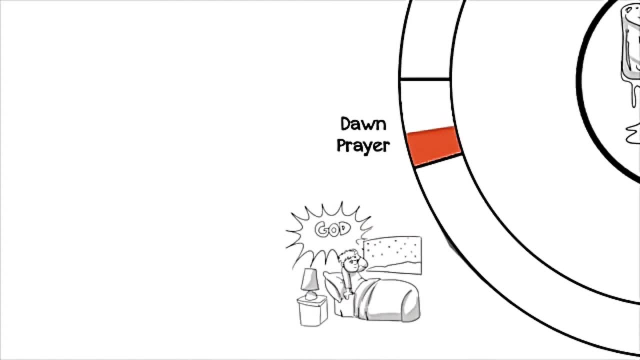 attaining spiritual happiness. Try to awake from sleep before dawn, a noble time, and let the first words in your heart and on your tongue be the remembrance of God. Purify your body and get dressed appropriately with the intention of obeying God. Pray in your home, then make your 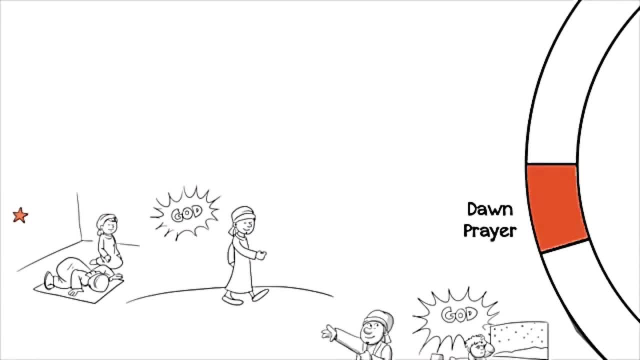 way to the mosque, in tranquility and with remembrance of God. Pray with the congregation, which is 27 times better than a prayer. Do not fail to complete this profitable act, for if you are negligent, then what benefit is there for you in the pursuit of knowledge? After all, the fruit of knowledge is enacting upon it. 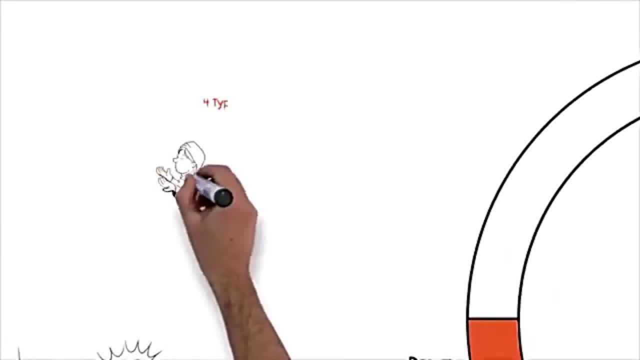 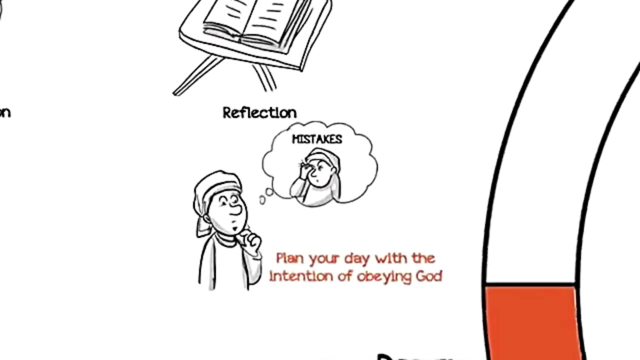 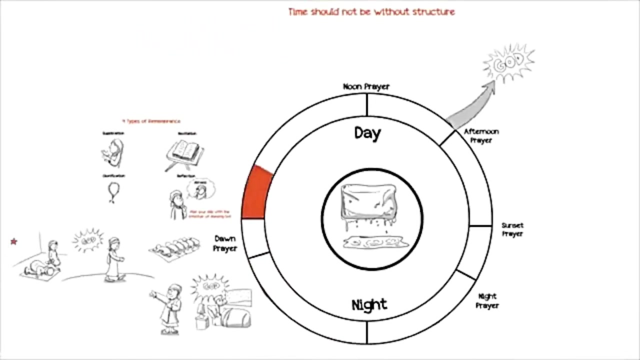 Use your time until sunrise in four types of remembrance: supplication, glorification, recitation and reflection. Reflect upon your mistakes and the nearness of your end and carefully plan your day with the intention of obeying God. By the light of day, you should strive to occupy yourself with what benefits you in the hereafter. 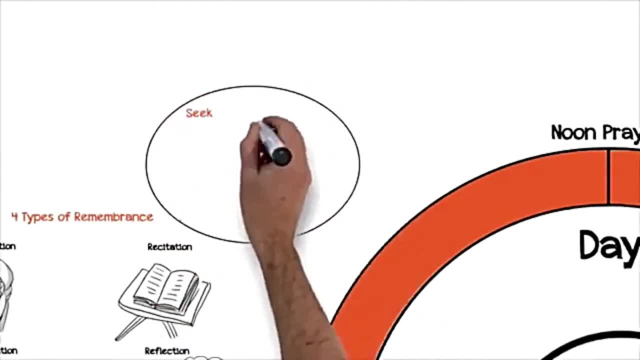 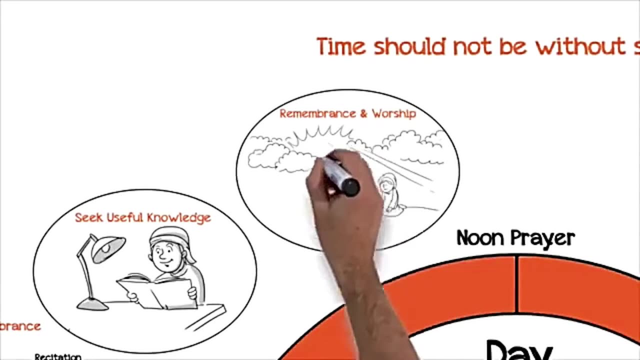 Use your time in one of four ways. The first is seeking useful knowledge. This is the best use of time and highest form of worship. Useful knowledge increases your God-consciousness. If you are unable to acquire useful knowledge, use your time in extra prayers. 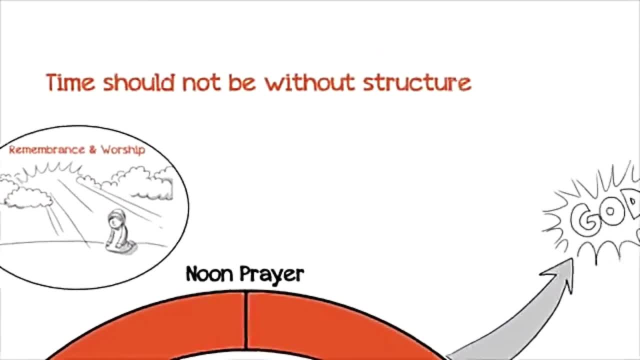 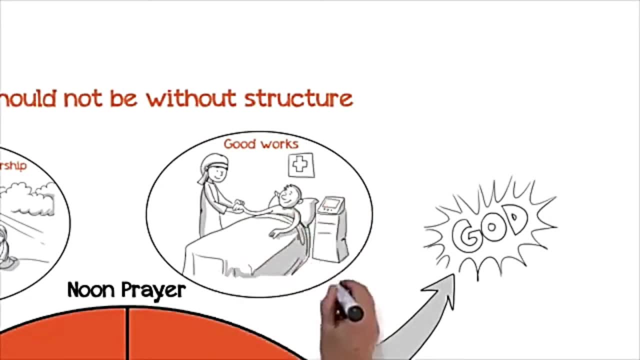 or one of the four types of remembrance mentioned. The third use of time is to act in a way that will bring happiness to the hearts of believers or make it easier for the righteous to accomplish good works, such as visiting the sick and feeding the poor. 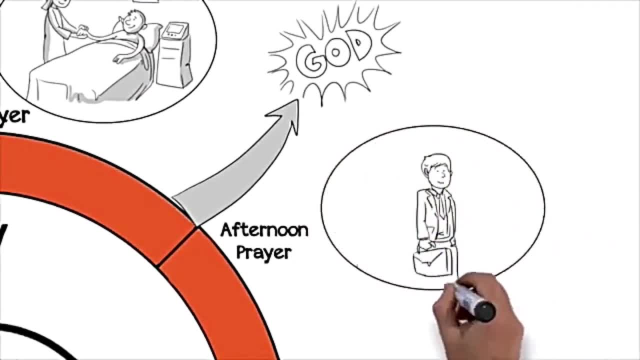 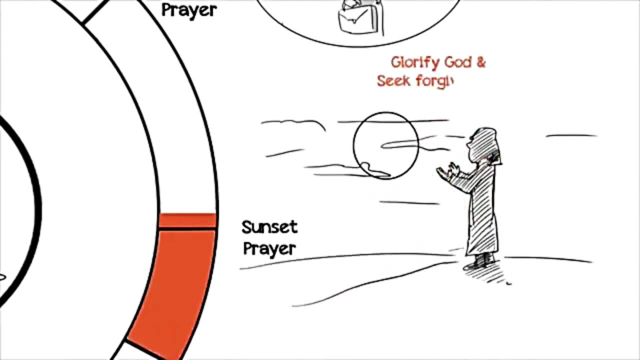 Finally, spending your time earning an honest living To take care of yourself and your family is also a form of worship. However, beware of worldly greed, for it will ruin your religion. When the sun turns red, try and spend your time glorifying God. 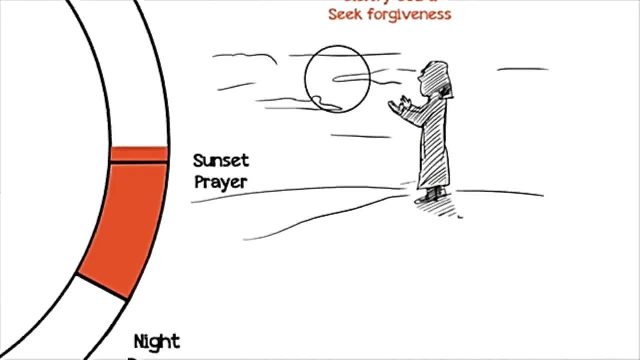 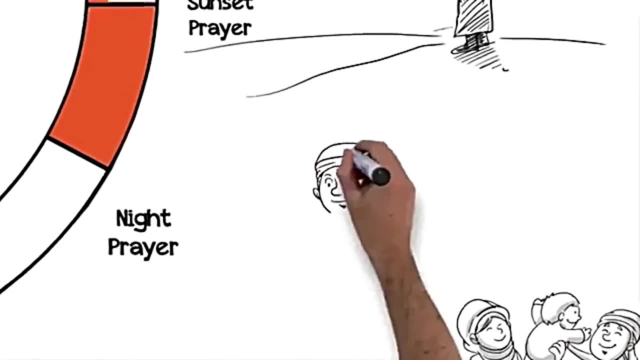 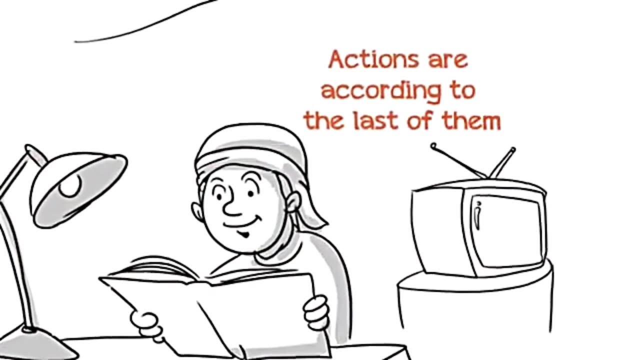 The sun should set while you are seeking forgiveness. One must also set aside time for worldly necessities, family and community. Before you sleep, review your knowledge. Do not end your day in entertainment, for actions are according to the last of them.